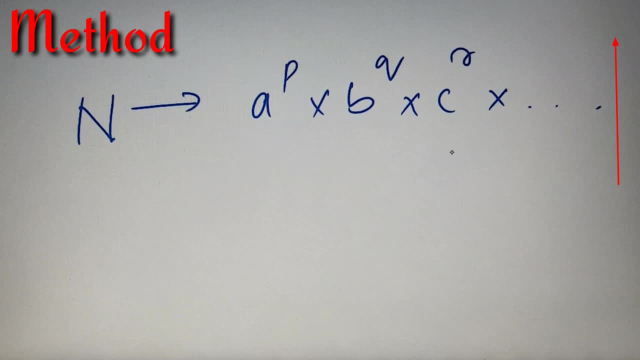 I have made a separate video on prime factorization so if you are still confused then you can go watch that video first and then come back to this video. So the number of factors which are perfect square for the case of n is equal to the integer. 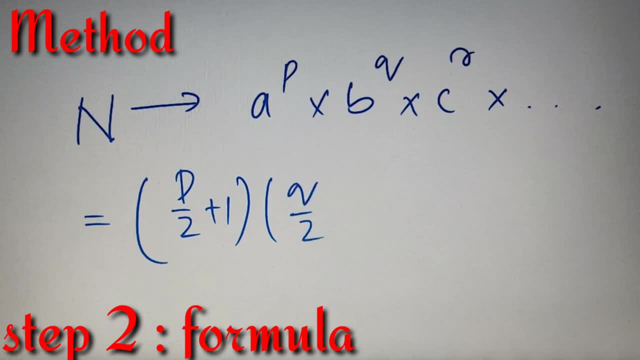 value of p by 2 plus 1, into the integer value of q by 2 plus 1, into the integer value of r by 2 plus 1.. Now, by saying integer value, what I mean is if the value in the bracket is equal to 10.5, then we will only take the value as 10 and 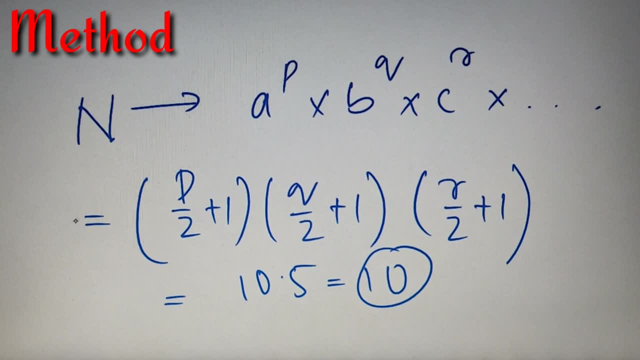 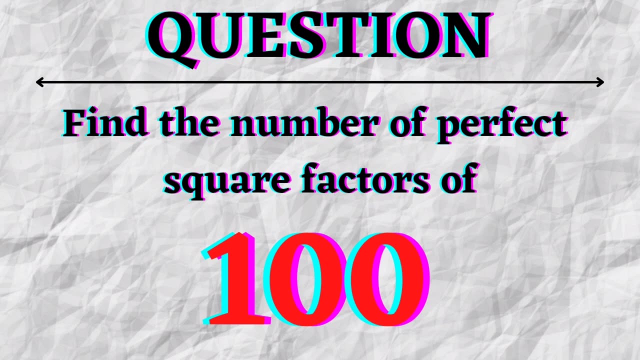 not as 10.5.. So by this simple formula, we can easily calculate the number of factors which are perfect square for the case of any given n. Now, according to our first question, we have to find out how many factors of 100 are perfect. 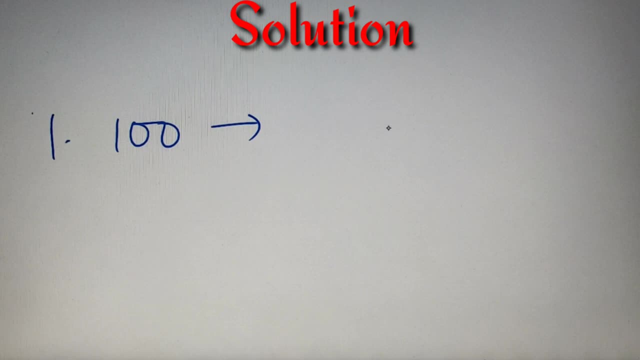 squares. Now, according to our formula, the first step is to prime factorize the number. Now we know that 100 is equal to 4 into 25, which can be further simplified as 2 square into 5 square. So the prime factorization of the number 100 is equal to 2 square into 5 square. 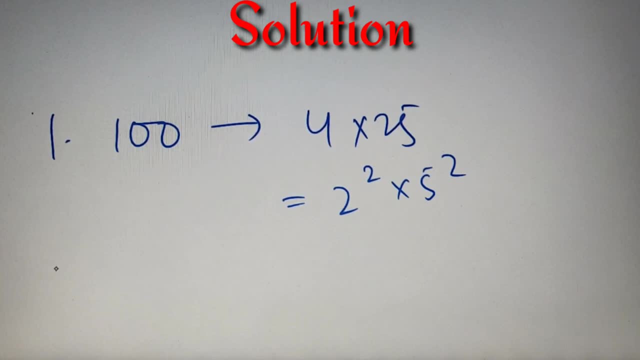 So we will just put the values 2 and 2 in the formula and we will get our answer. So the value that we have to calculate is equal to the integer value of 2 by 2 plus 1 into the integer value of 2 by 2 plus 1.. 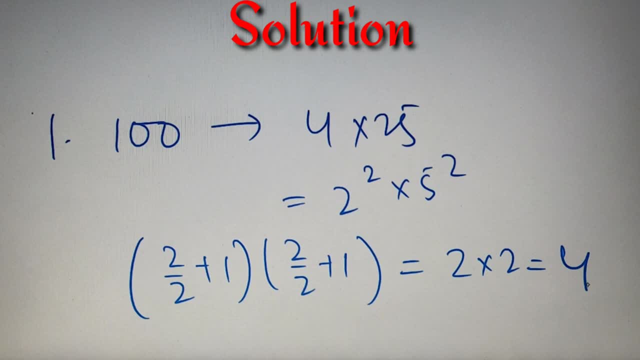 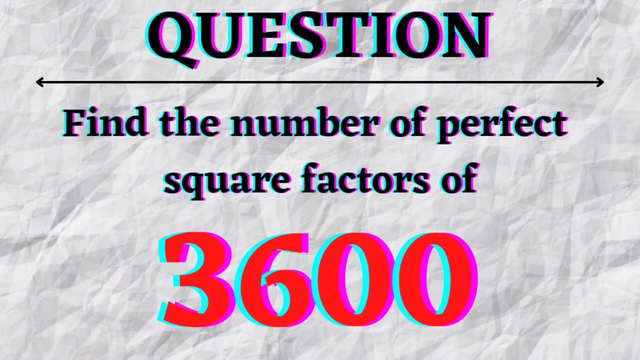 Now this value is equal to 2 into 2, which is equal to 4.. So the number of factors which are perfect square, for the case of 100, is equal to 4.. Now, according to our second problem, we have to find out how many factors of 3600 are perfect. 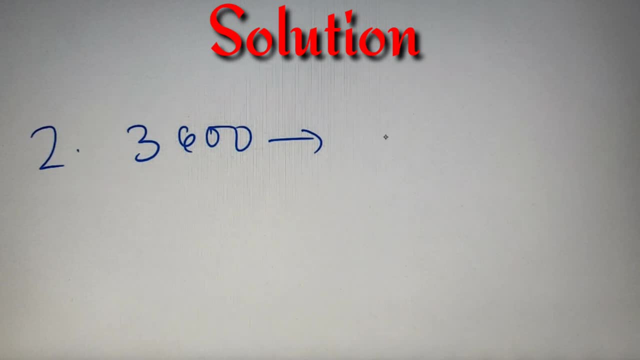 square. Now, first we will prime factorize this number. Now, 3600 can be simplified as 36 into 100, and we know that 36 is equal to 6 square, which is equal to 2 square into 3 square, and we know. 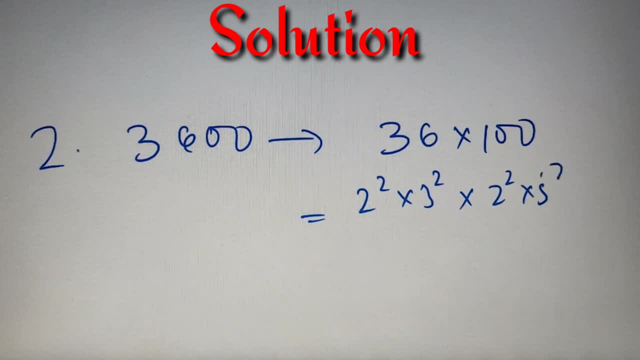 that 100 is equal to 2 square into 5 square. So the prime factorized form of 3600 is equal to 2, to the power 4 into 3, square into 5 square. Now this is the fastest way to prime factorize the. 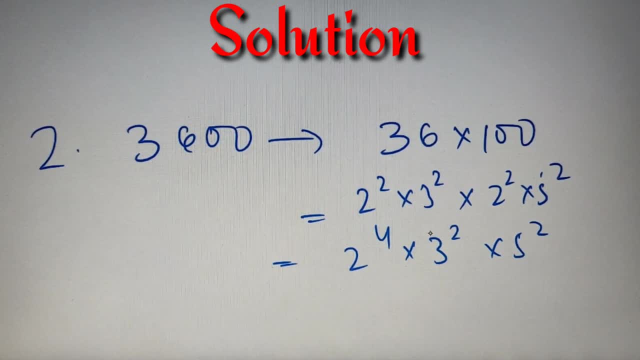 number, and I would recommend that you should also follow this method as well. So in putting the values in the formula, we will get the integer value of 4 by 2 plus 1 into the integer value of 2 by 2 plus 1, into the integer value of 2 by 2 plus 1, which is equal to 3, into 2, into 2, which